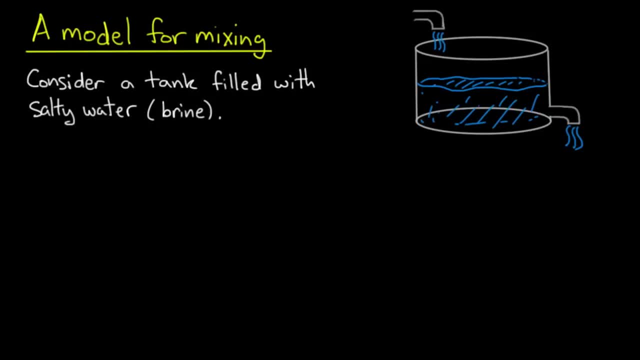 When you study a certain kind of differential equation, for example a first-order linear differential equation, it's often helpful to have in mind a physical system which would be modeled by that differential equation. So I'll introduce now a model for a mixing process, and this mixing process will be modeled by a first-order linear differential equation. 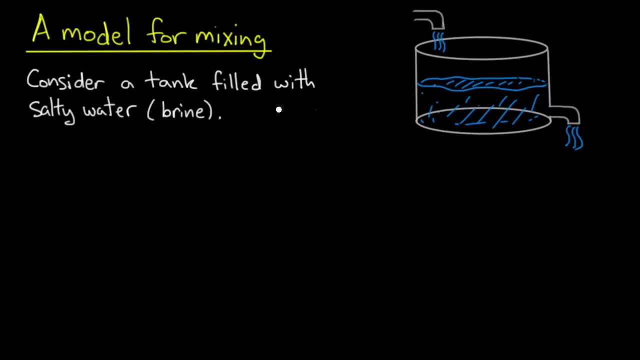 So suppose that I have a tank full of salty water. I'll call it brine. Now into the tank is flowing more brine and, depending on the problem, it might be saltier or less salty or the same saltiness. Now out of the tank is pouring a perfect mixture of what's in. 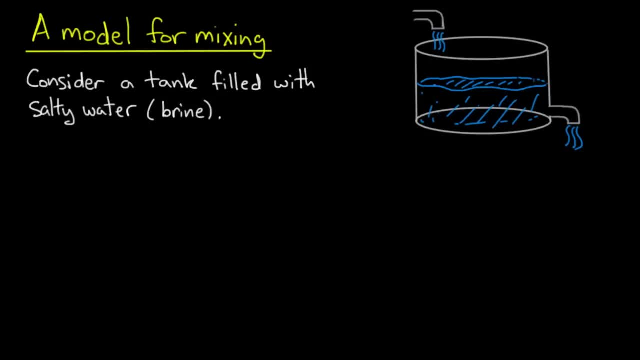 the tank already and what's pouring into the tank Now? let's quantify all of these things. So let's say that the brine flows into the tank at a rate of R? in and it has a concentration, a salt concentration, of C in And the brine flows out of the tank. 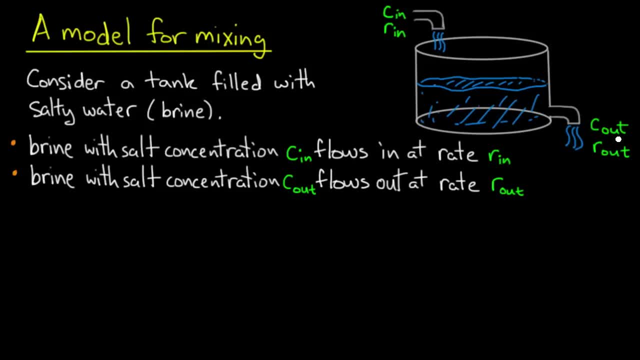 at a rate of R out And it has a concentration of C out. Let's give names to two more quantities. Let's call X the amount of dissolved salt in the tank, So the total amount of salt dissolved in this brine, And let's call V the total. 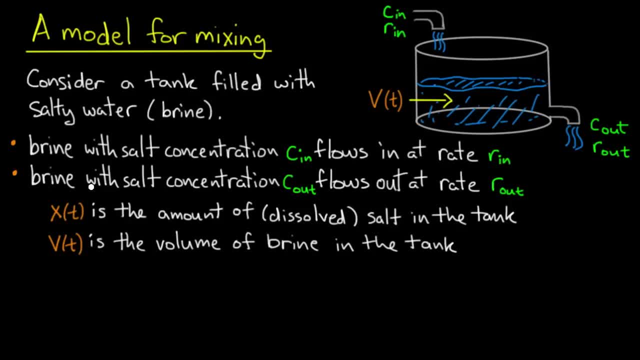 volume of the brine. Now these two quantities are changing in time. V, for instance, may be changing if the rate in is different from the rate out, And X will of course be changing because mixed brine is flowing out meanwhile other brine maybe saltier or maybe less salty. 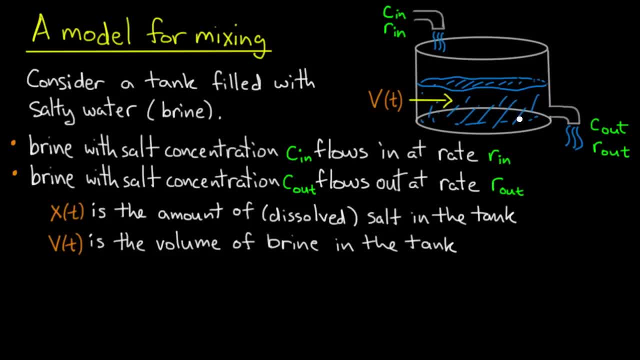 is flowing in, So the total quantity of salt in the tank will be changing. Our model will be a model for the amount X of dissolved salt in the tank, And we will find that it is a first order linear differential equation for X. Now how could we come up with such a model? Well, let's consider a small time interval. 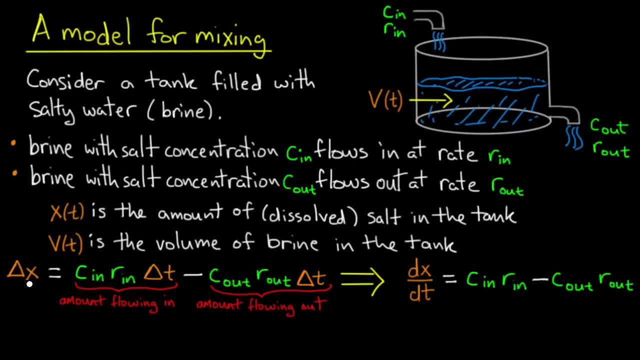 and let's try to write down what the total change in the amount of salt is over the small time interval�: JS, SNG, You can call that delta X. Well, what is delta X? How does the In dunes lot of time interval haya dangerous is without the 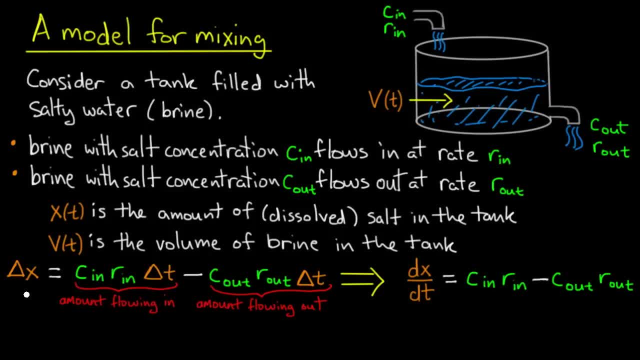 change over for delta t. Well, in a tiny time interval, a certain amount of salt flows in and a certain amount of salt flows out, But it's not too hard to deduce that the total change in the amount of salt will simply be the amount of salt flowed in minus the amount that flowed out. Now how would we know? can't really tell for certain, but if we had the two different terms also in common then I wouldn't worry about the other terms. figures Simple enough to figure out that salt there won't change over the entire amount of salt In one last example: the low dissolve rate in 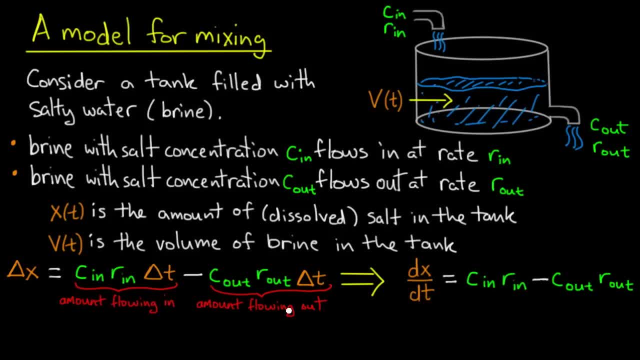 that flowed out. Now, how do we determine how much flows in and how much flows out? Well, we know the rate at which brine flows in and we know the concentration of salt in that brine. Knowing these two quantities, we actually know the rate at which the salt flows in. 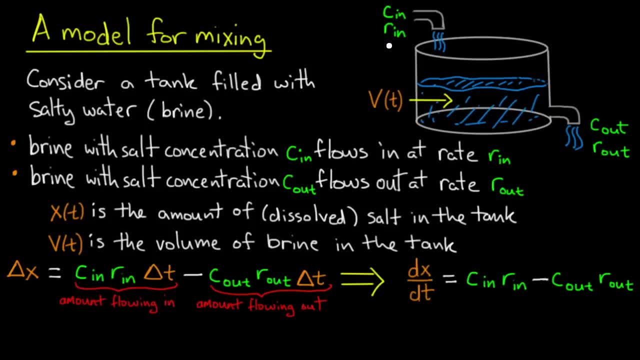 It's C in times R in. For example, if the rate in is one gallon per minute and the concentration in is one gram per gallon, then the rate at which salt flows in is C in times R, in which is one gram per minute. So same goes for the rate out, So the rate of salt. 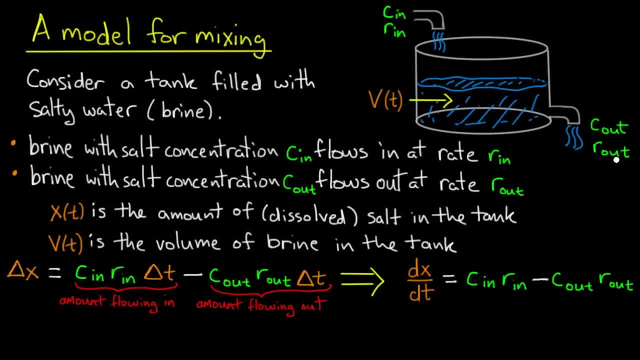 flowing out is C out times R out. So we know the rate at which salt flows in and we know the rate at which salt flows out. So how do we figure out the total amount of salt that flowed in and the total amount that flowed out over the time interval delta T? Well, 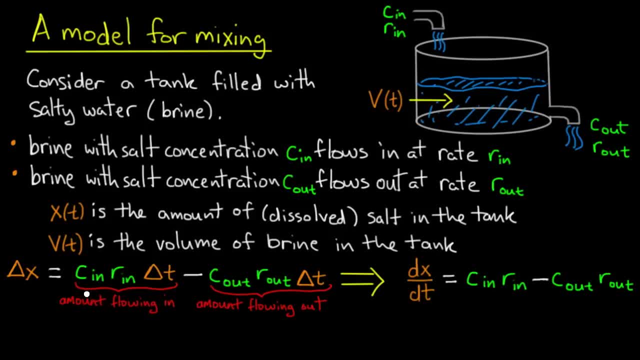 we multiply by delta T, So the total amount of salt that flows in over that small time interval, delta T, is C in times R in times delta T, and we subtract the total amount that flowed out during that time interval, delta T, which is C out times R out times delta T. Now, this is not yet. 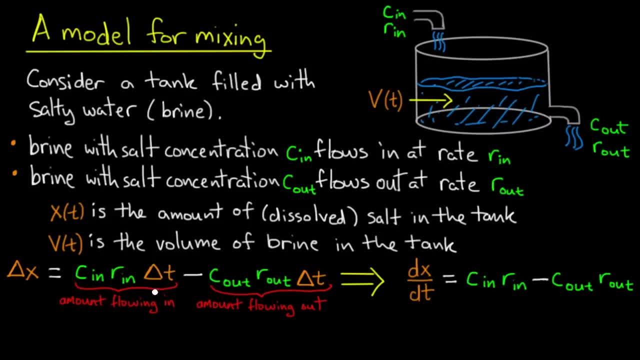 a differential equation. But we're considering a little tiny time interval, delta T, So we can turn it into a differential equation by dividing both sides by delta T and letting delta T go to 0. So taking the limit as delta T goes to 0. So that quantity delta X divided. 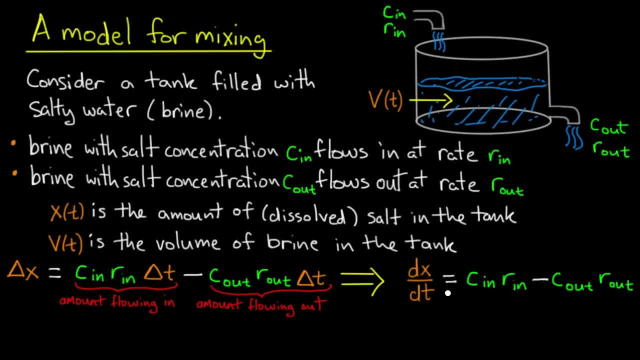 by delta, T becomes dXdT And dx dt is equal to C in times R in, minus C out times R out. Now what we've got here looks pretty good, but it doesn't look like a differential equation yet. On the left-hand side I have dx dt and on the right-hand side I have these funny things: C in, R in, C out, R out. 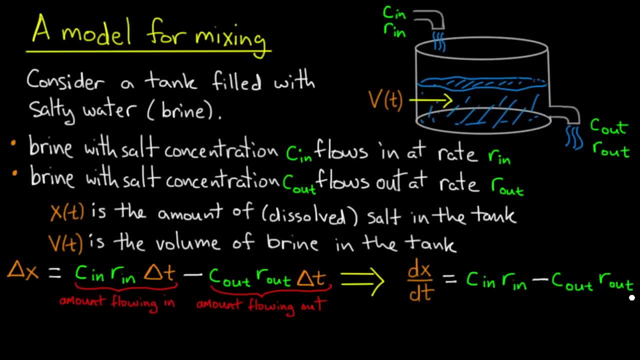 So let's see if we can make this look like a differential equation, And to do that, let's consider the following question: What quantities on the right-hand side do you control and which do you not control? So let me explain what I mean.